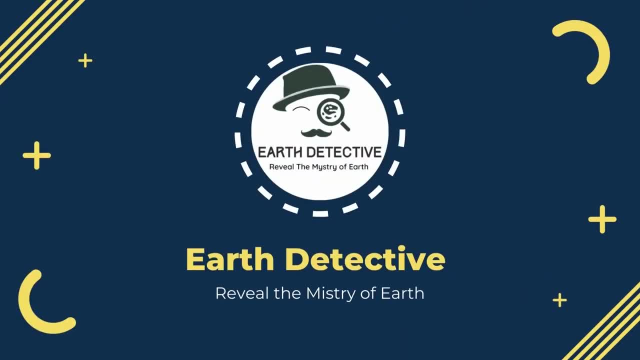 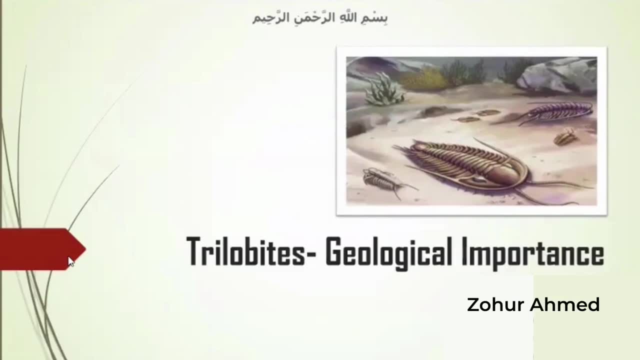 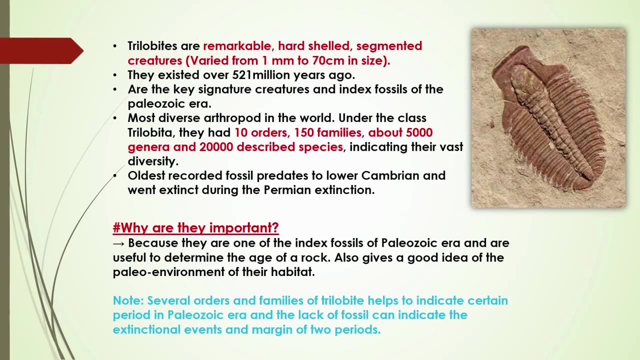 Assalamu alaikum, I am Johor Ahmed. I welcome you all to this presentation about the geological importance of trilobites. Without any further ado, let's start our presentation. Firstly, what is trilobite? It is a hard-shelled creature with segmented body parts which roamed around the 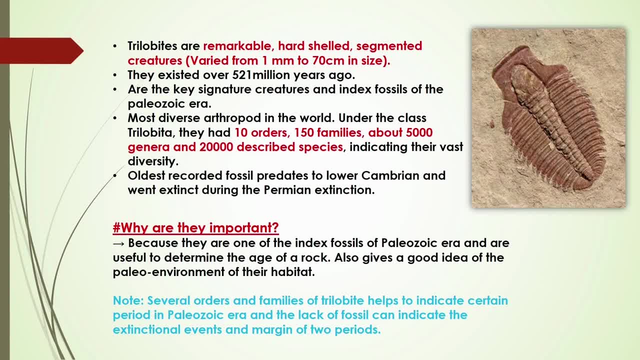 world during the Paleozoic era. They were about 1 millimeter to 70 centimeter in length, depending on the species, and were very diverse around the whole world. They were so diverse that under the trilobite class there were 10 orders, 150 families, about 5,000 genera and over 20,000 described. 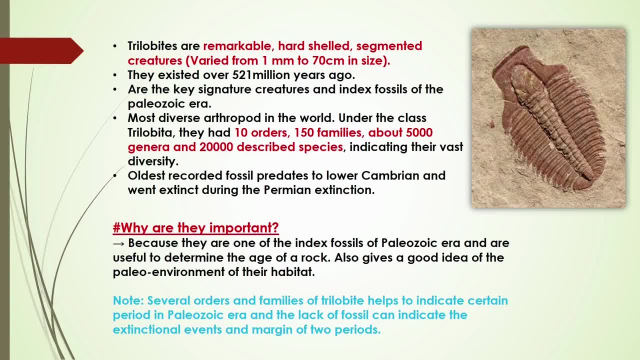 species. Now, why has this extinct arthropod become so important in geology and geological history? Well, they are one of the most important index fossils of the Paleozoic era, which helps us to determine the age of particular strata. The lack of this arthropod fossil in the Paleozoic 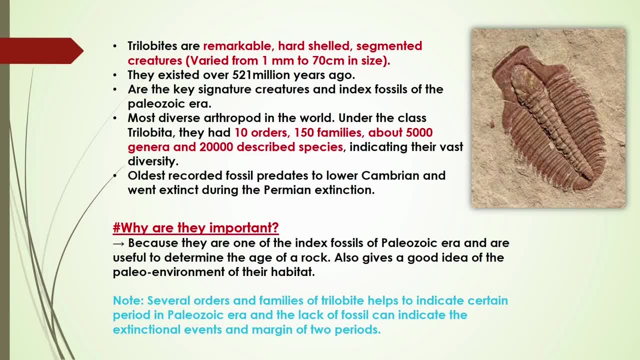 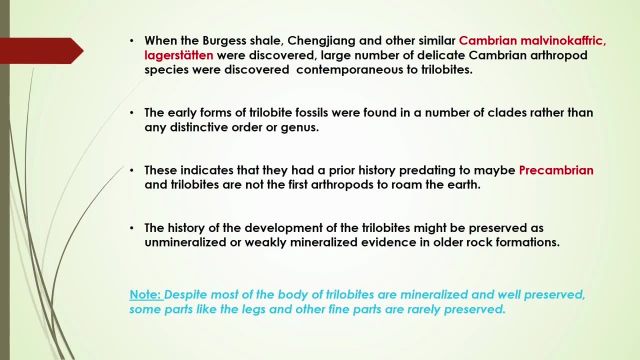 formation also indicates various extinction periods. It is used to believe that the trilobites were the first arthropod on the earth, but new fossil evidence found in Cambrian Malvinographic Lagustatine hints that the way there were more ancestors of the prehistorical arthropod. 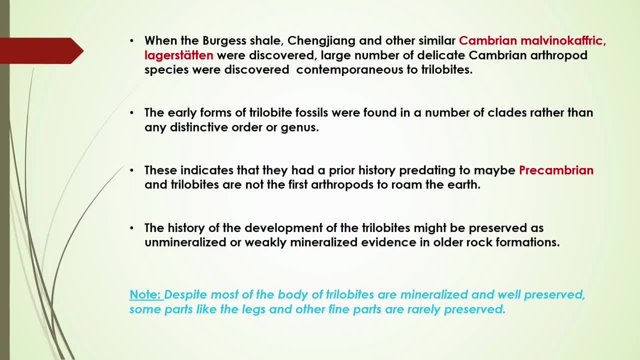 dating back to pre-Cambrian, which might not be as well fossilized as the trilobites. Thus, more and more trilobite fossils are found in the Paleozoic formations. Despite being well fossilized, the fossil record does not preserve soft parts of the trilobite body. 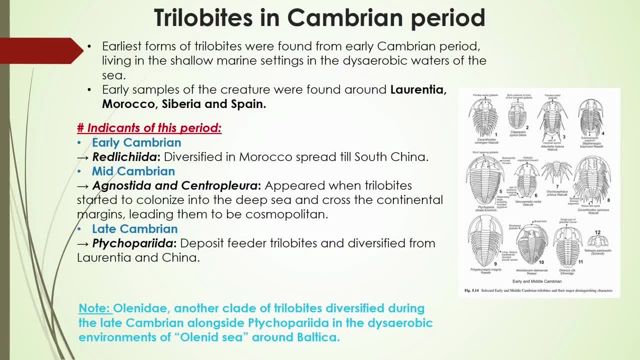 The first of the trilobites is believed to be from the early Cambrian. The species in this period are believed to be shallow marine dwellers found in Laurentia, Morocco, Siberia and Spain. The period is divided into three timelines: early- mid. 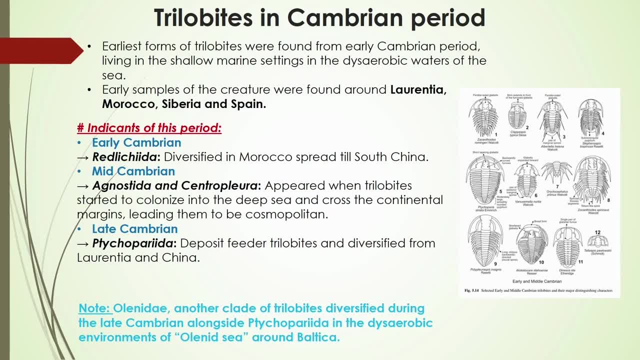 and late Cambrian. Early Cambrians saw the diversification of trilobites, namely Retlichida spreading across Morocco to south China. Agnostida and Centovisoridae started colonizing the deep waters. This enabled these trilobites to diversify all over the world. in the mid Cambrian, 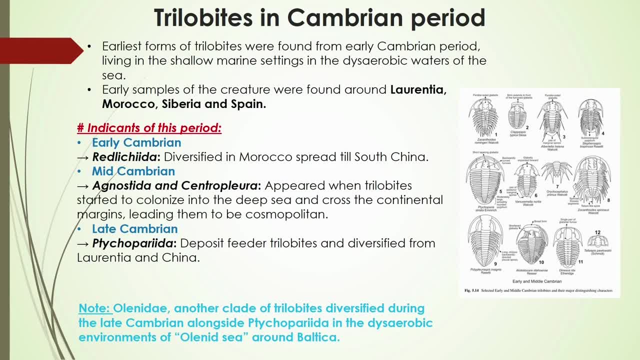 In the late Cambrian. Tychoperidae was abundant in Laurentia and China, alongside Olenidae, another clade of trilobite in the Olenets Sea, around the Baltic paleocontinent, which is equivalent to the present-day Eurasia. 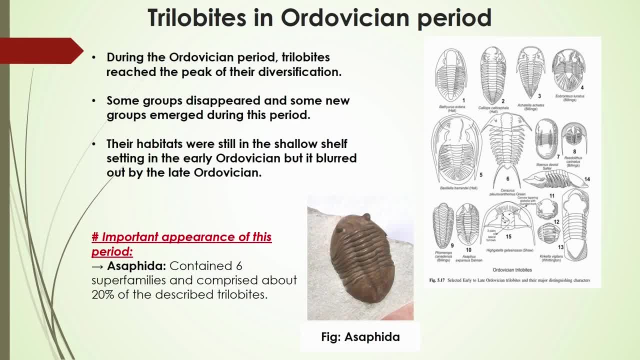 In Ordovician they reached their highest point of diversification. Shallow water provenance was still seen in Ordovician, but in the late Ordovician they began to disappear. An important appearance of this timeline is Asaphida, comprising of 20% of the described. 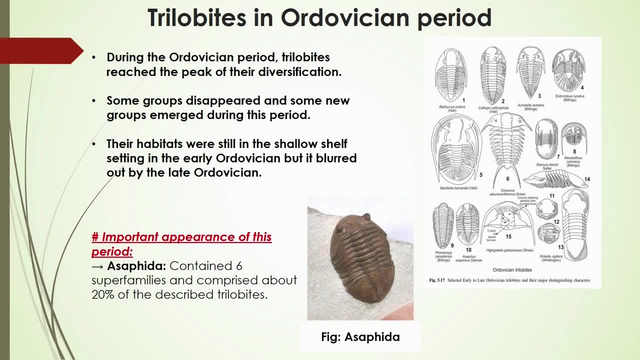 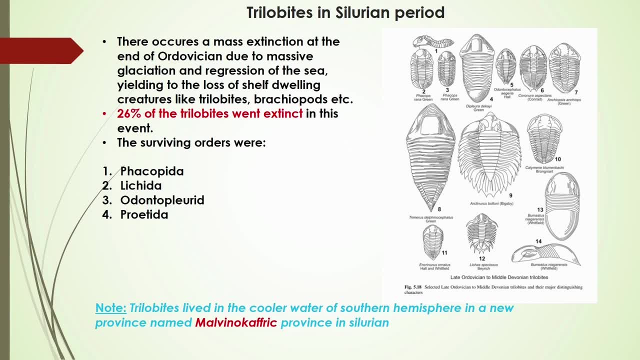 trilobites and containing six superfamilies. In the Silurian period, the trilobites faced a massive extinction due to the massive regression of the sea due to glaciation. 26% of the trilobites died in this extinction. 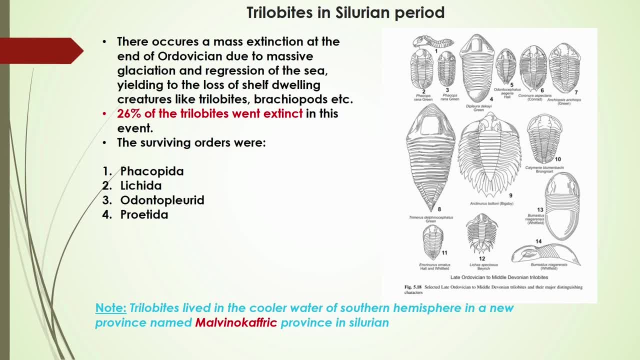 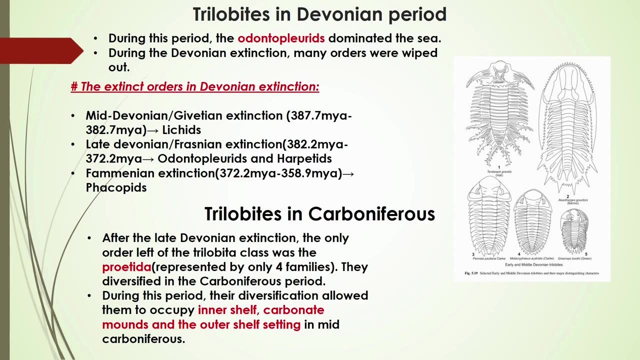 Order surviving were Phacopita, Lychida, Odontoplurite and Proteta. They moved their habitat to the southern hemisphere in a new province called Melvinopolis. Most of the orders in the trilobites went extinct in the Devonian period and the Odontoplurites 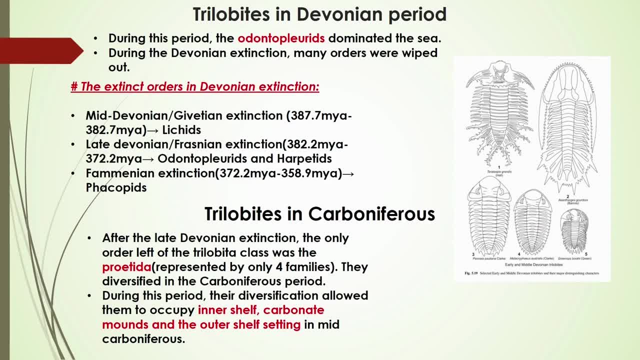 dominated the sea in this period. The Gevassian or the Mid-Devonian extinction wiped out the Lychids. Late Devonian extinction wiped out the Odontoplurites and the Harpetids, and the Feminine extinction wiped out the Phacopites. 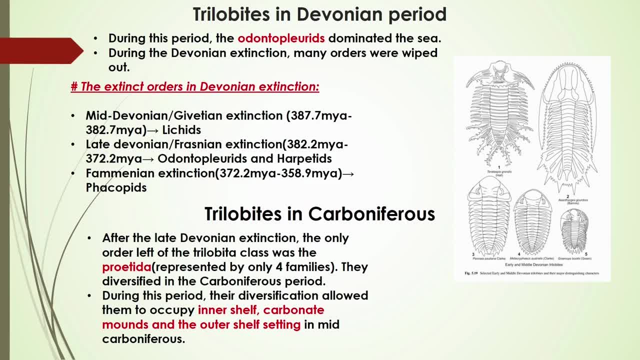 After the late Devonian extinction, the only living trilobites were the Proteta, represented by only four families which diversified in duration. The Proteta was the only living trilobite in the inner shelf, carbonate mounds and 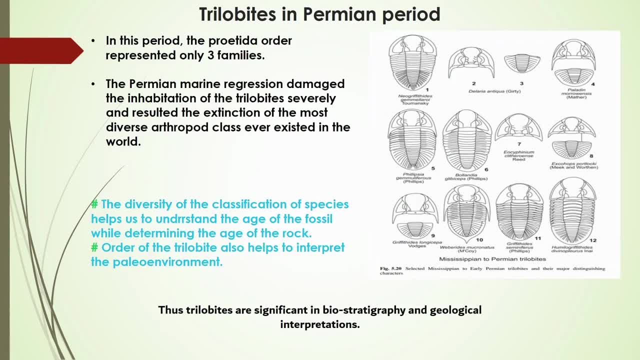 the outer shelf region. Finally, after surviving through several extinctions, the Protetes went extinct in the Great Permian extinction due to the regression of the sea which damaged their habitat. As we can see from the previous discussions, characteristic orders of the trilobites lived. 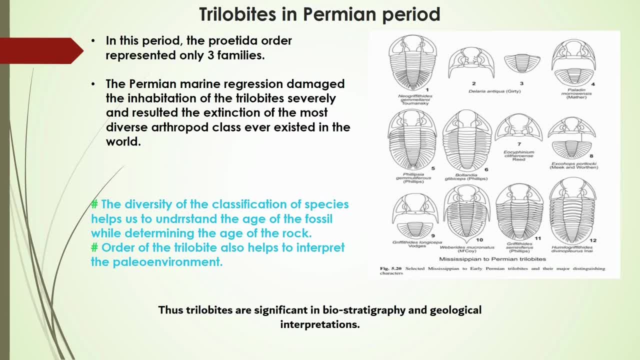 in different periods in Paleozoic era, which is very useful information to determine the age of the Paleozoic formation. Moreover, the habitat of the index trilobite is very crucial data to depict the Paleoenvironment. This allows us to date a formation on a broad scale, even without isotope dating method.